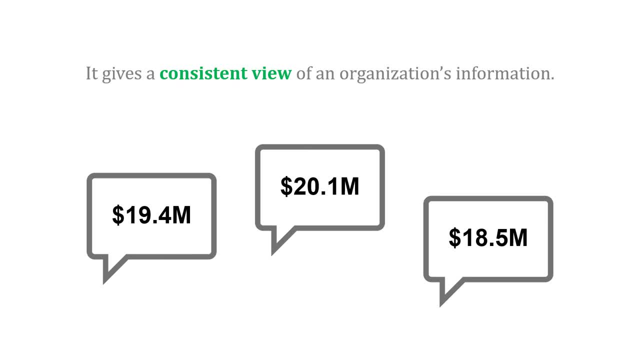 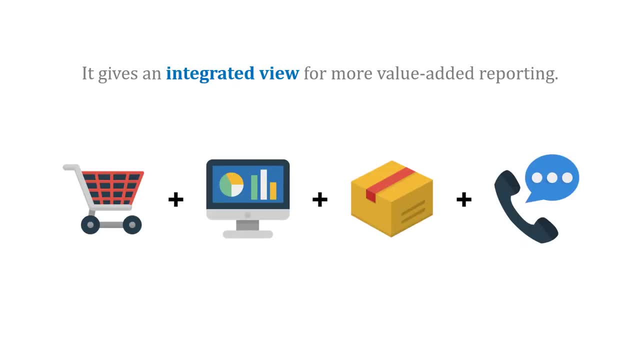 off the same sheet of music. What you don't want to do is go into a meeting and have different numbers for revenue. You want to have a consistent, consistent set of information. Additionally, that data warehouse gives an integrated view for more value-added reporting. So, for example, it can give us a more complete view of our customer. 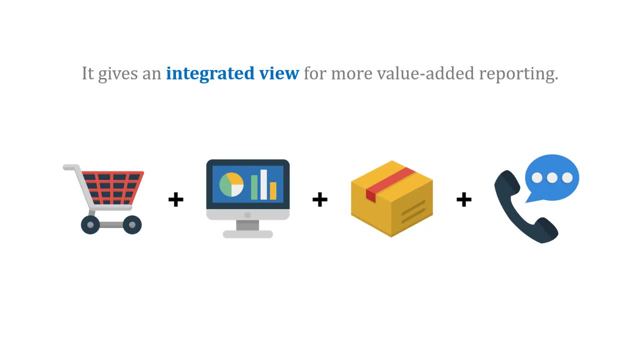 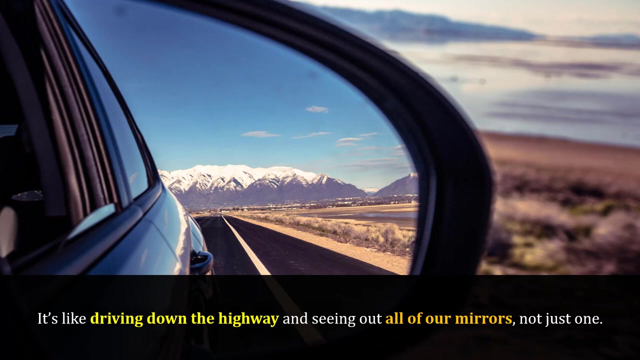 so we understand maybe support calls that they have shopping data, shipment data. It brings it all into one place so we can better understand that customer. It's kind of like driving down the highway and seeing out of all of your mirrors and not just one, You get a more full picture of. 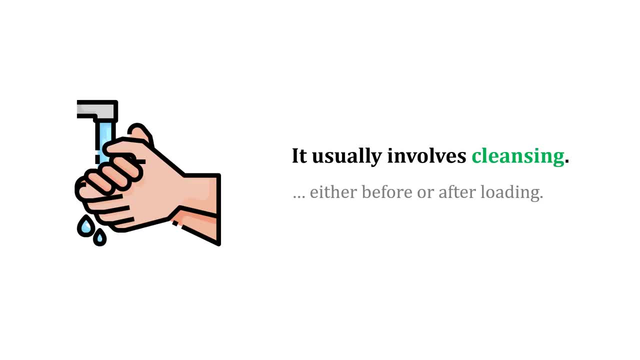 your business or of your customer in our case. Also, when we're bringing data into the warehouse, it often needs to be cleaned, either before or after loading. As a couple of examples, we may remove duplicates, which can be common when we combine data sources. 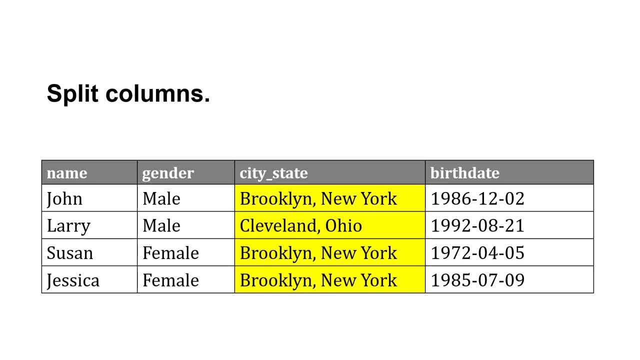 Also splitting columns, for example, splitting the city and the state in this scenario, or filtering out irrelevant observations which aren't important for our analysis. Now, when we perform this, we're going to be able to do a lot of things. We're going to be able to do a lot of things. 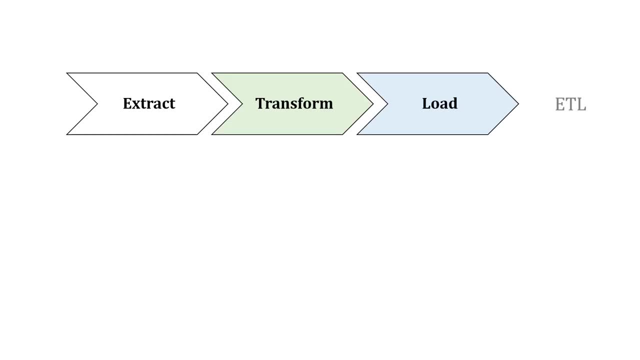 and we're going to be able to perform this cleaning or this transformation. When we do that, before we load it into our data warehouse. that's known as an ETL process. We extract the data, we transform or clean it and then we load it. Another way of doing this is doing the loading and then the 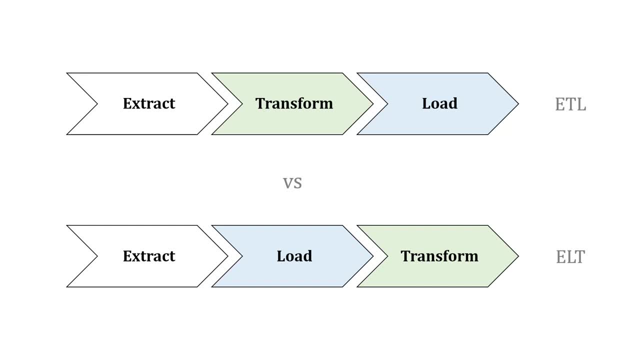 transformation. That's ELT, So we extract the data, we load it into the warehouse and then we perform the transformations while it's there. So we could be using ETL or ELT. Additionally, the tables inside the data warehouse can be organized in a variety of ways. 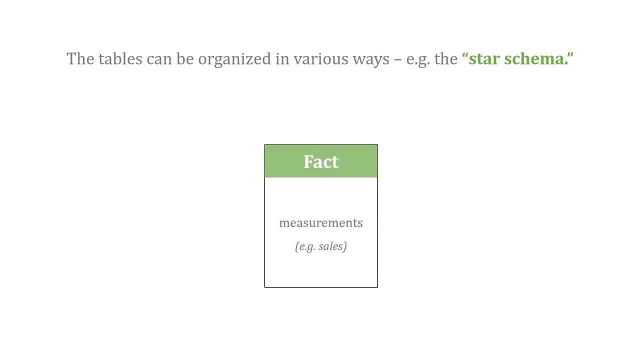 Probably the most famous is the star schema, where at the heart of it you have a fact table with measurements like our sales data, And then around that fact table you have supporting dimensions which provide more context to those measurements or the sales, like a list of 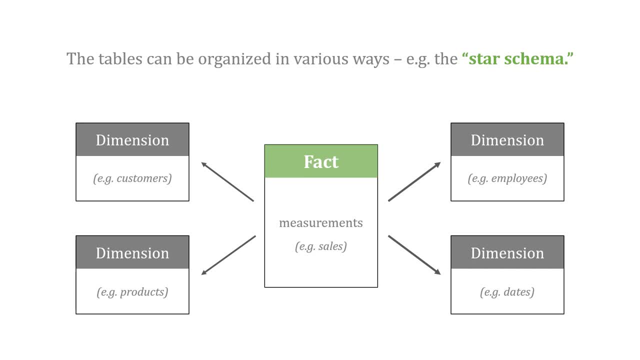 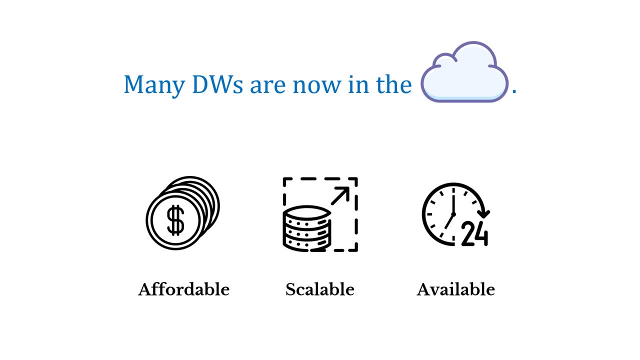 customers, employees, products or other things. And finally, many data warehouses are now moving into the cloud For a few reasons. The cloud is affordable. You pay as you go or only pay for what you use. It's scalable. You can grow those data warehouses really quickly And they're available. There's